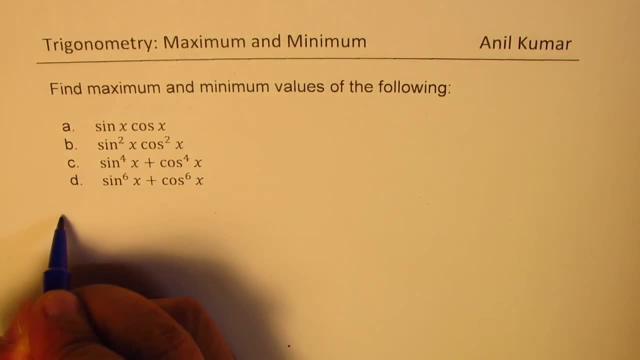 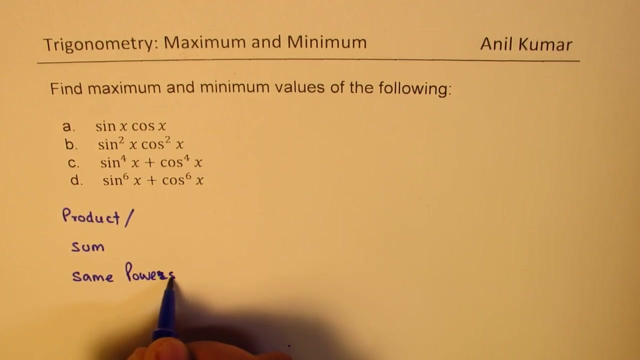 here is: we have a product or we have sum, right. However, in all the cases we have same powers, Correct? So let us see how to get maximum minimum value for such cases, right? That's the whole thing. Then in the next video, we'll take different powers. 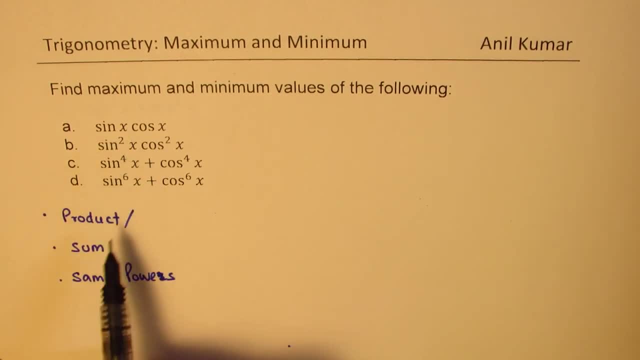 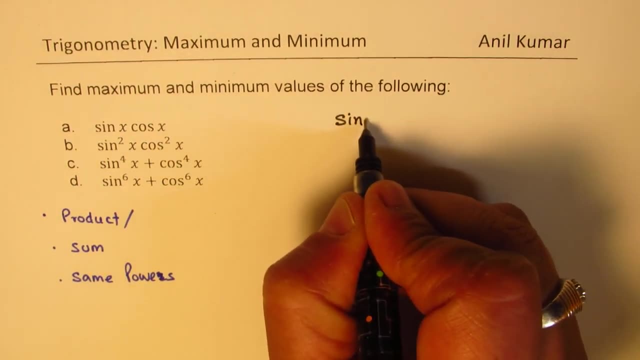 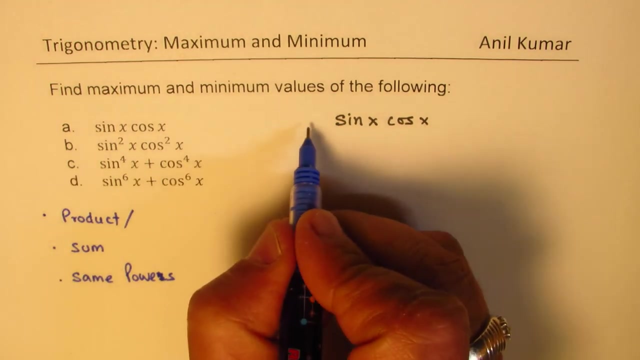 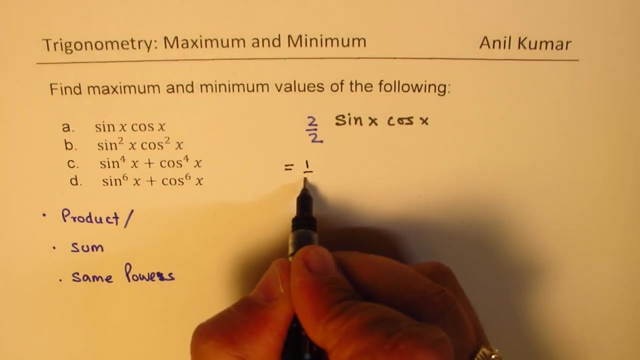 Even and odd will make huge difference. Now to understand this, let's understand sine x, cos x, the base function, first, right. So when I say sine x, cos x, I could always multiply and divide by 2 right. So we could multiply by 2 and divide by 2.. So that means I could always write this as half of 2 times sine x. 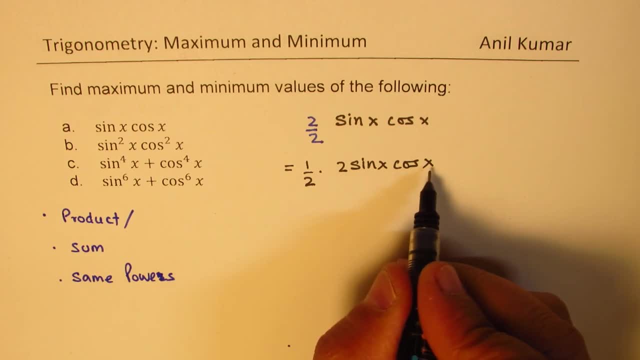 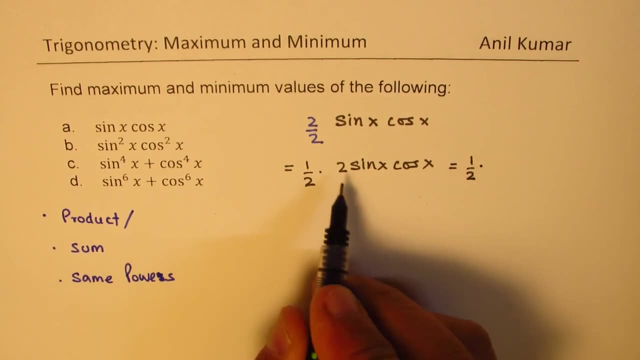 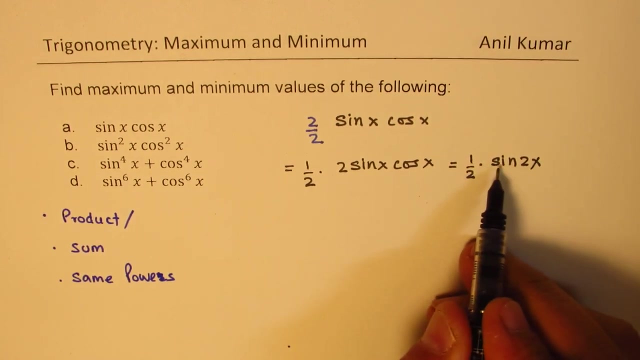 cos x. Now 2 times sine x. cos x is sine 2 x. So this can be written as half of 2 times sine. cos x is sine 2 x. Now that becomes a sinusoidal function which will have a maximum and minimum right. So, as you can see, that sine 2 x. 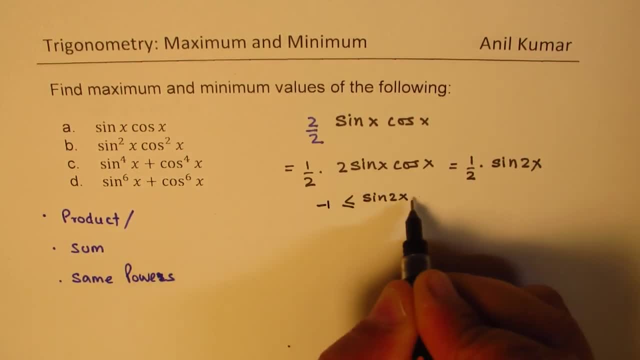 will have a value which will be from minus 1 to plus 1, right? So if I do half of this, so I get minus half. half of sine 2 x to plus half. Is that clear to you? So that is the maximum minimum value. 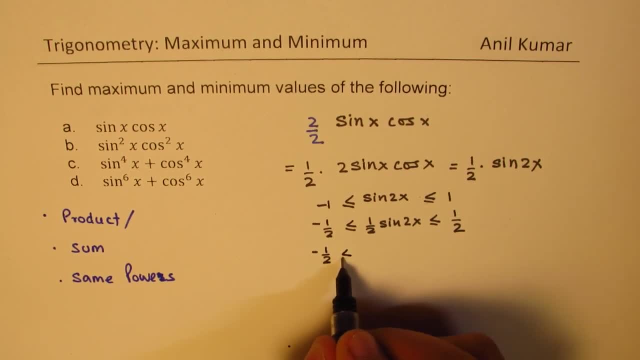 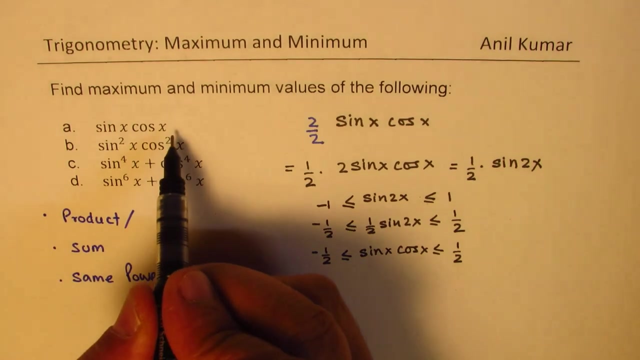 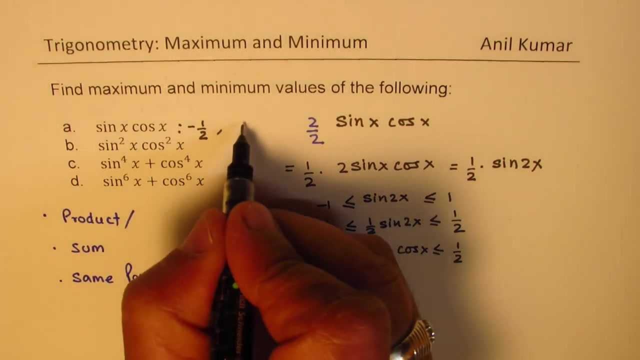 for your function sine x cos x, which is also same for sine X Cos X, right? so I'm showing it like this so that you try to understand that. how are we going to do this, right? so so, for the first case, we got the minimum value as minus half and the maximum value is plus half. so this is. 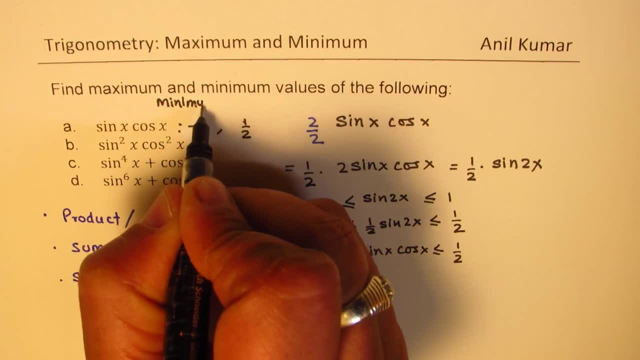 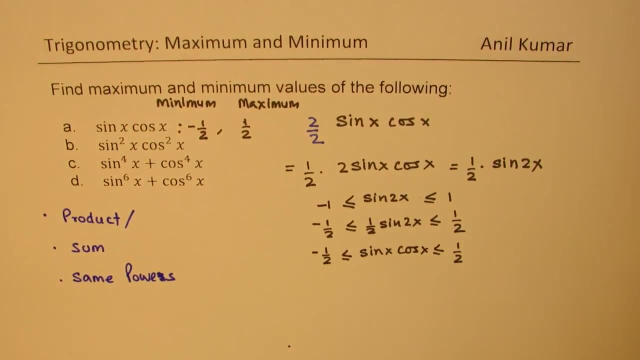 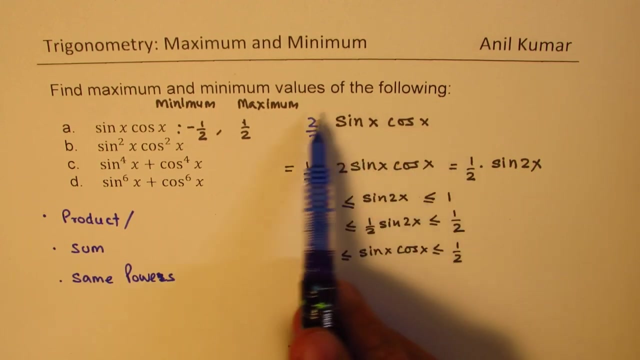 your minimum, and that is your maximum, perfect. now, if you're working with square of this, right, then what happens? well, if you have square of this, we basically have to square this up, whatever we were working with right. so when we have sine square X, cos square X, in that case we will have to multiply. 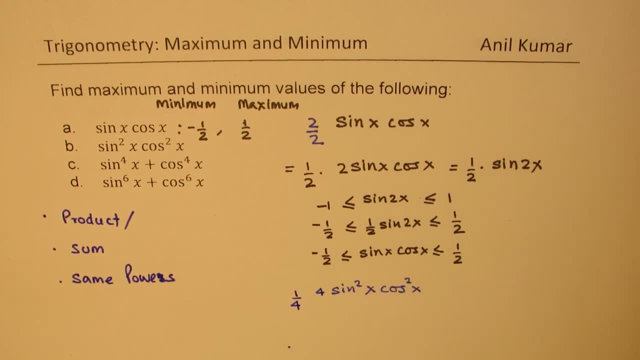 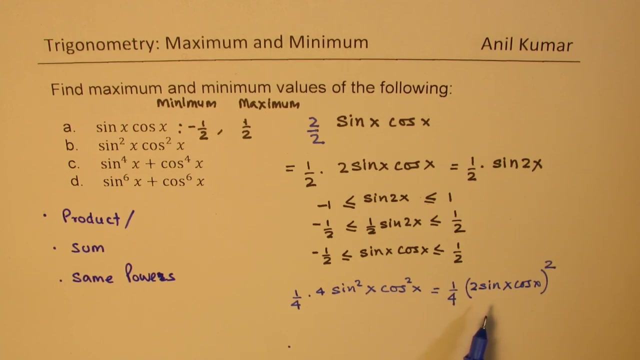 and divide by 4. right, correct. we have to multiply and divide by 4, and so this could be written as 1 4th of. think like this: 2 sine X cos X, whole square. perfect now, force to sine x cos X, whole square. we could write this as equal to 1 4th of sin 2 X whole. 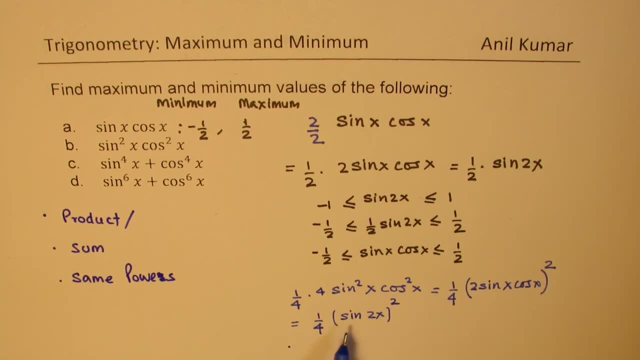 square. so earlier we found that for sine 2 X, which is between minus 1 and 1, and now this is 1 fourth of that correct. so so in this particular case, sine 2x, whole square will always be positive. see, it's kind of important to understand that when we square the value, it is always going to be. 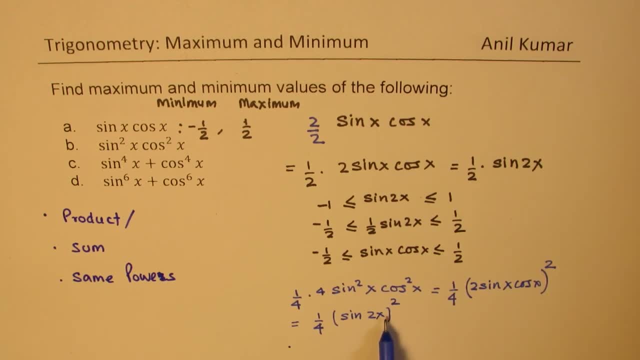 positive right, so it will never be negative. so in this case the minimum value will be 0, right, not negative right, so so in this particular case this value could be between 0 and 1, correct? so here what we will notice: that for this particular function, the value will be: 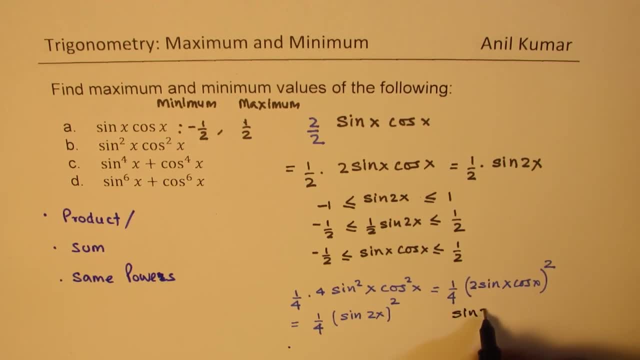 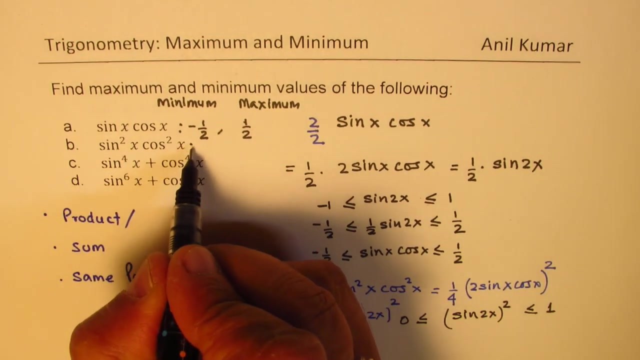 uh, let me write down: sine 2x whole square will actually be between 0 and 1, correct, because it cannot be negative, perfect. and therefore if i multiply by 1, fourth, then that minimum value will be 0. so for here the minimum will be 0. however, the maximum 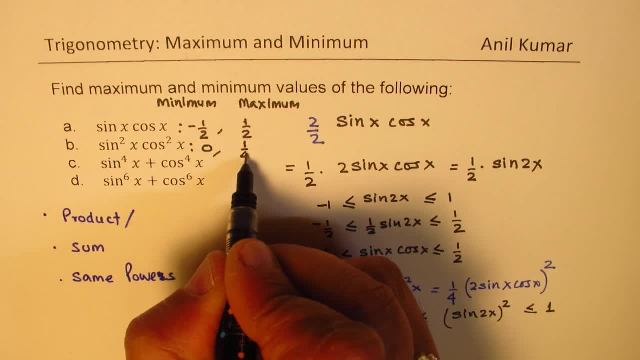 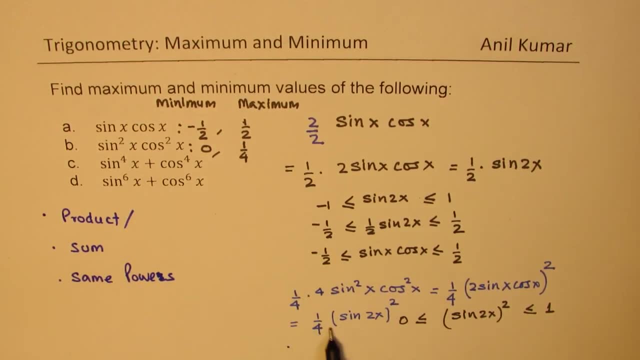 will be 1. fourth, which is 1 by 2 whole square. do you notice that correct? so so that is how we are going to get the maximum minimum values for these. so i hope this is absolutely clear, right, so we have done first and the second one. let's move on and take the case when we have some of 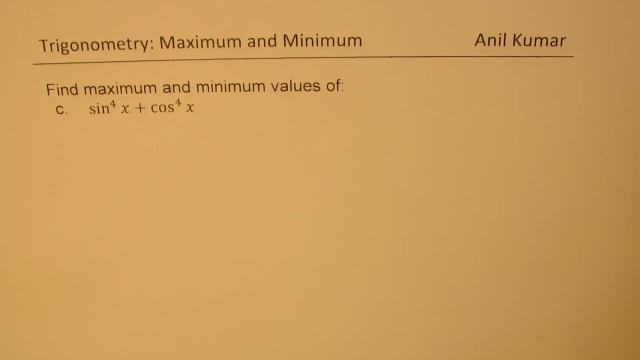 these. okay. so now we'll take sine to the power of 4x plus cos to the power of 4x and see what can we do in this particular case. now, if we have sine to the power of 4x plus cos to the power of 4x. 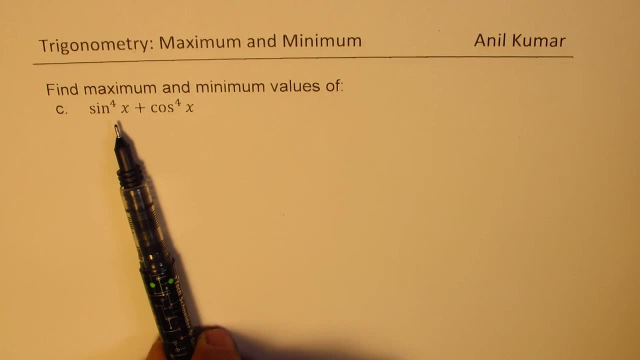 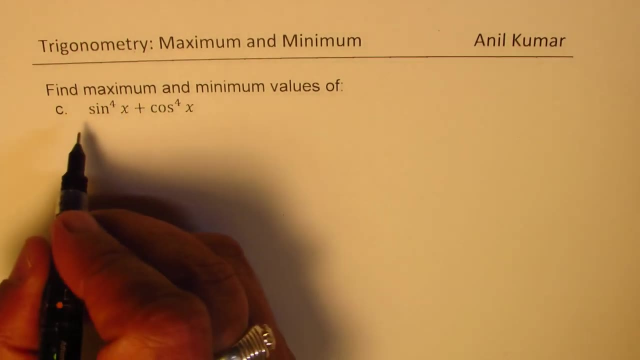 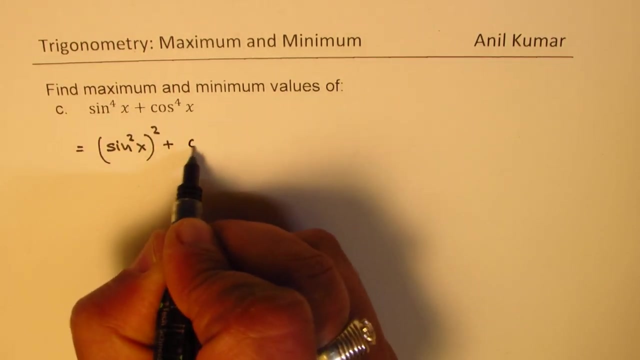 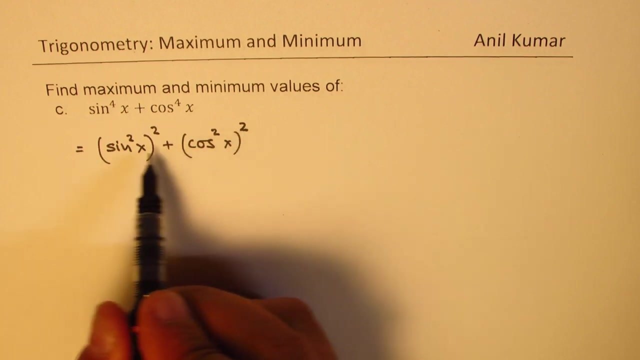 and cos to the power of 4x. we could write this as equal to sine square x whole square plus cos square x whole square, correct? so you write this as a plus a square plus b square. a plus b whole square, minus 2 a b, right? so it could be written as: 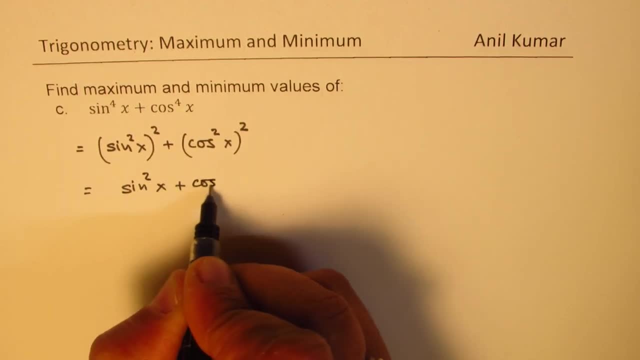 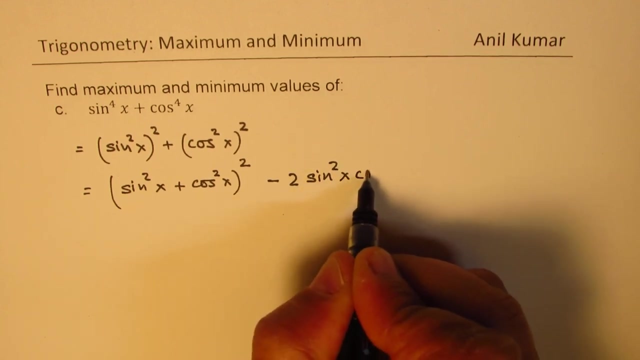 sine square x, plus cos square x, whole square. so you'll get the term these two plus 2 a, b. so we'll have to subtract that. so minus 2: sine square x, cos square x. now this term here is equal to 1, so we get 1 minus 2. 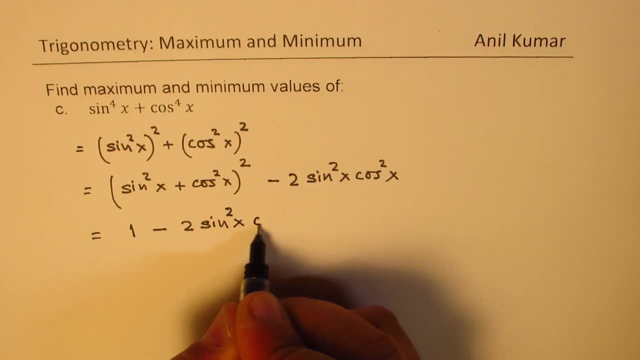 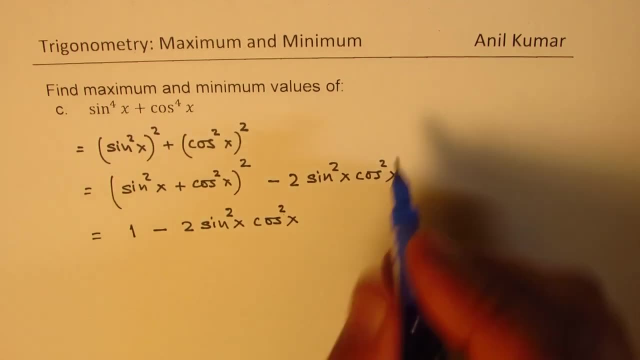 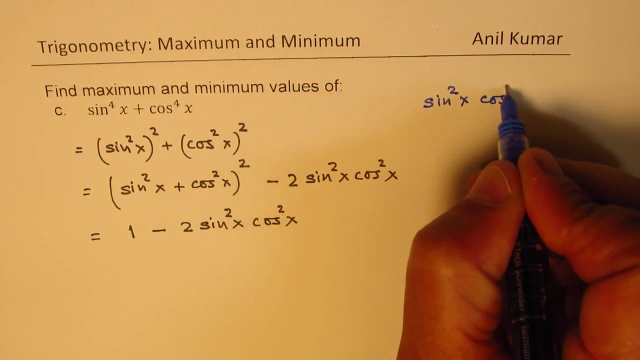 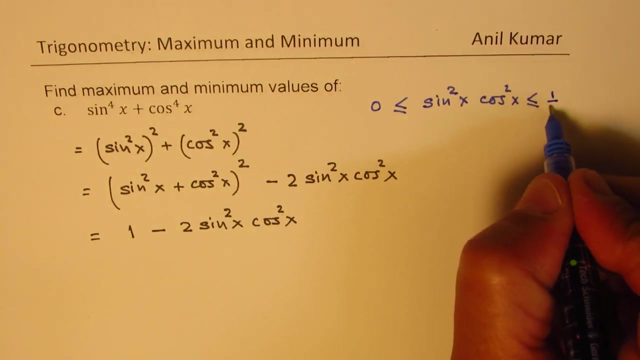 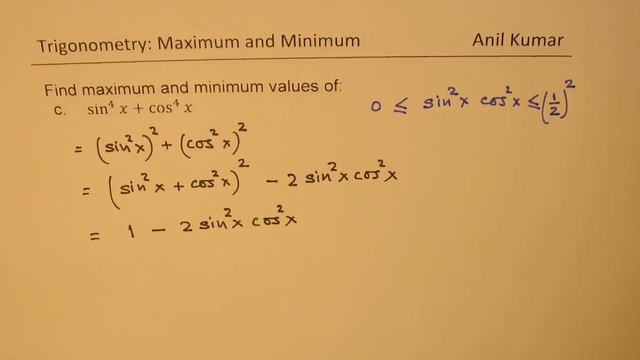 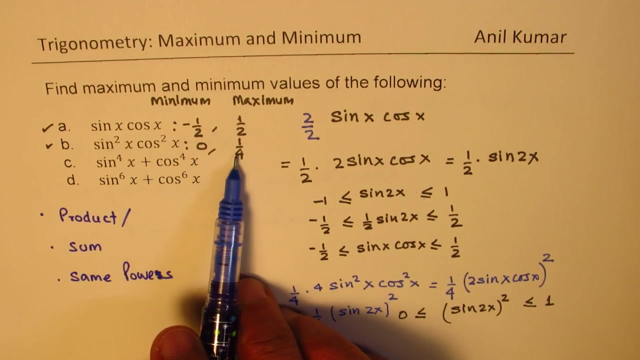 sine square x cos square x. correct now, we just saw that the value of sine square x cos square x is between zero and half square right. okay, we just saw that. so so earlier we saw that the product Sine square S cos square X was between 0 and 1 fourth, that is half square right. 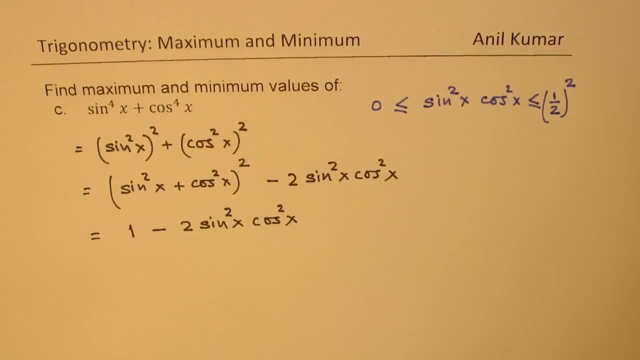 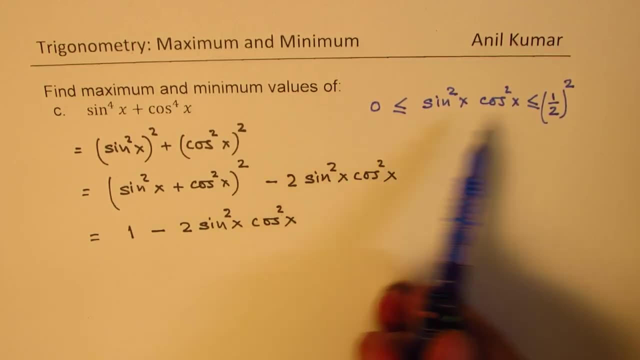 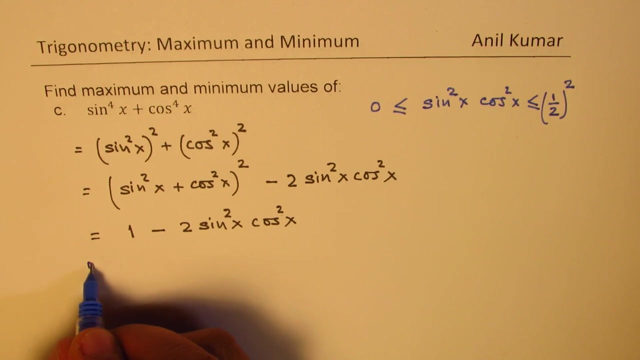 Now for getting the maximum value of this. we know this limit is between 0 and 1 by 4.. So here the maximum will be when you deduct the minimum right. So the maximum will be equal to 1 minus 0, which is 1.. 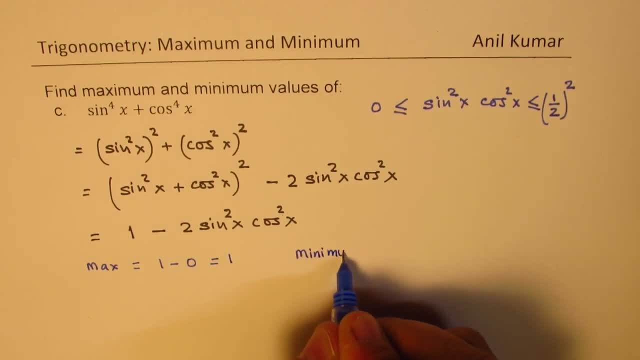 And the minimum will be when you take away the maximum, correct? So it will be 1 minus 2 times maximum for sine square X. cos square X is 1 over 4, right? So the minimum value is 1 minus half or is equal to half, right? 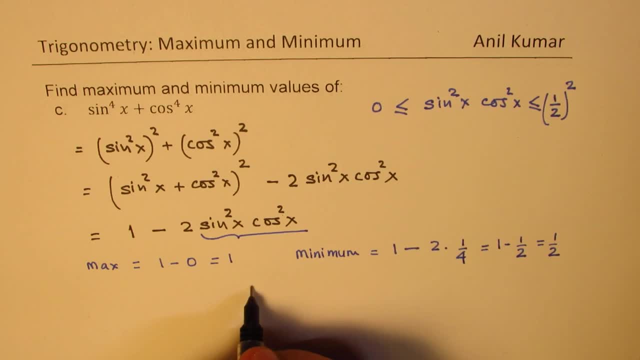 So for this particular function, we now know that sine to the power of 4X plus cos to the power of 4X will be between 1,. it will always be half right. Greater than equal to half. that is the minimum value. 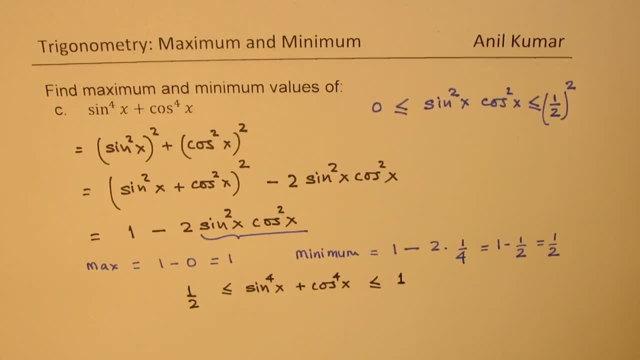 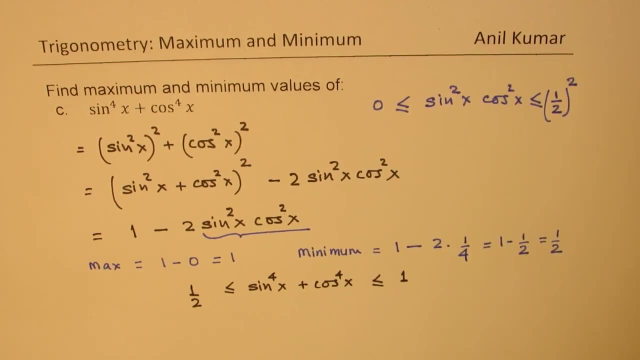 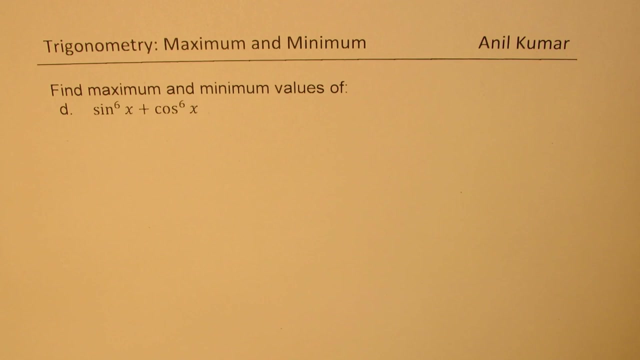 And it will be always less than 1, right, Less than equal to 1.. So that becomes the value for sine to the power of 4X plus cos to the power of 4X, correct? Now let's see the last example here, which is sine to the power of 6X plus cos to the power of 6X. 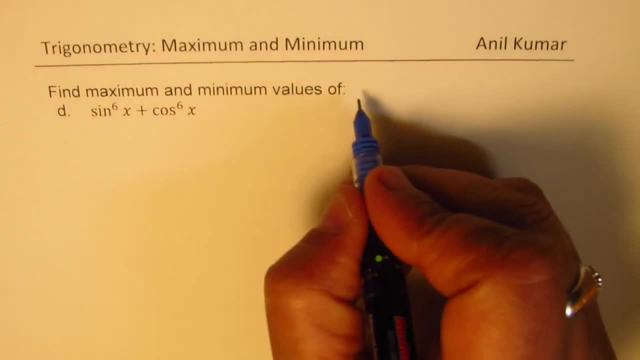 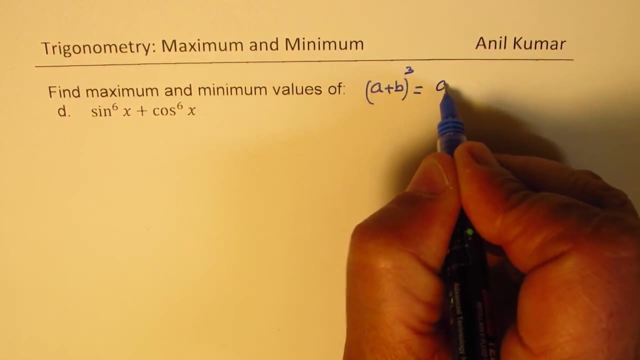 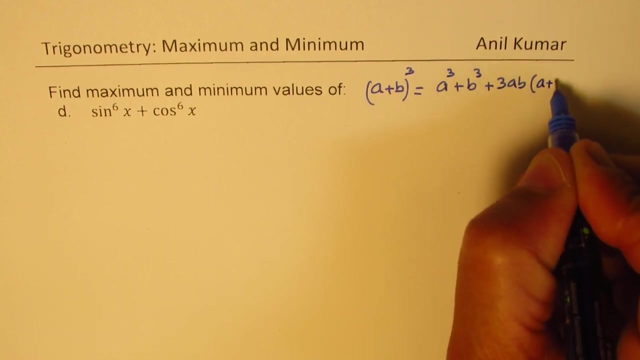 Now to work with the 6 powers. let us try to understand the A plus B whole cube formula right. So we have A plus B whole cube, which can be written as A cube plus B, cube plus 3AB times A plus B. 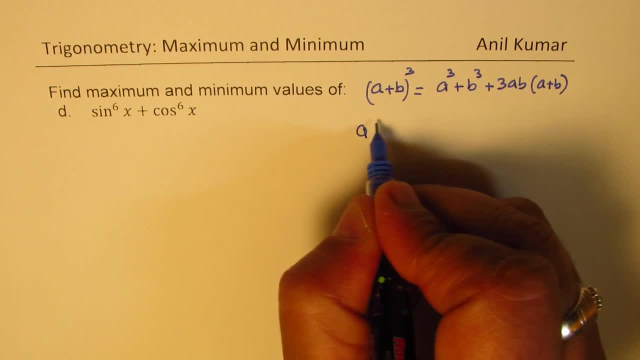 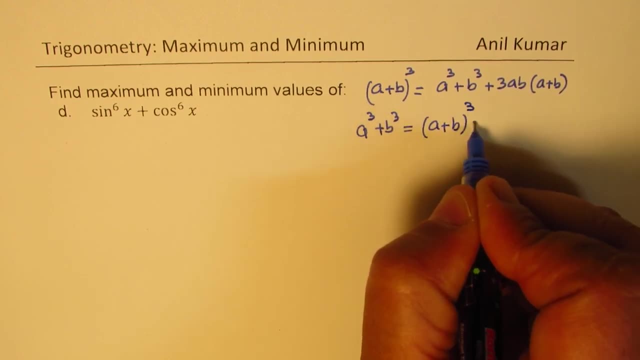 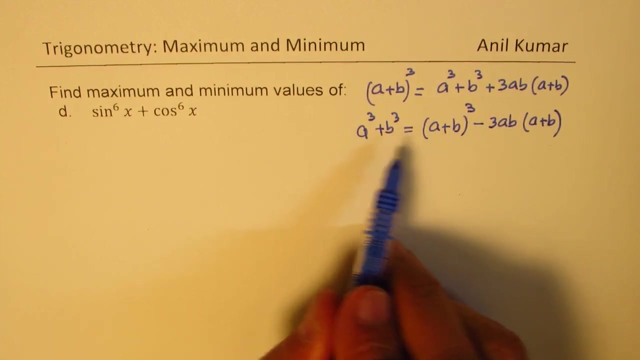 right. So from here we can rearrange And write down: A cube plus B cube equals to A plus B, whole cube minus 3AB times A plus B, correct? So we are going to use this formula to simplify the given expression. 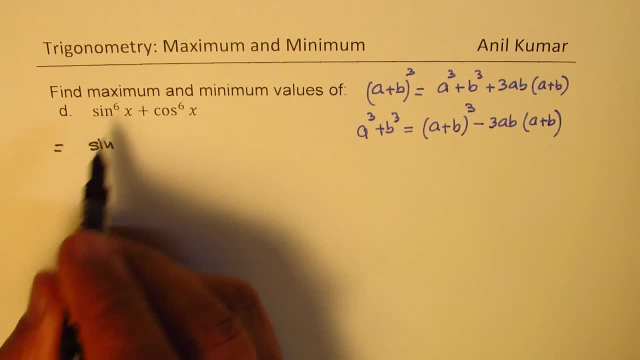 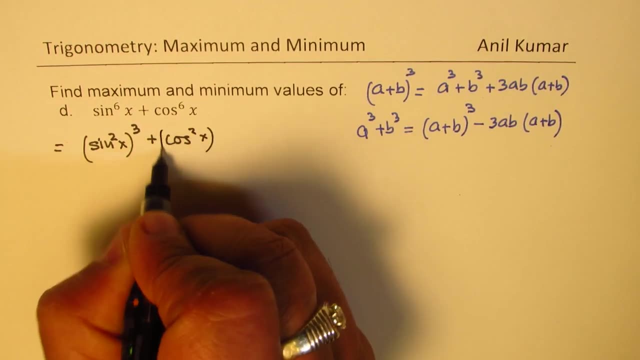 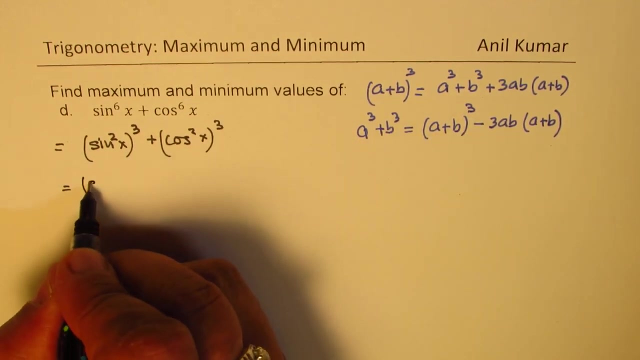 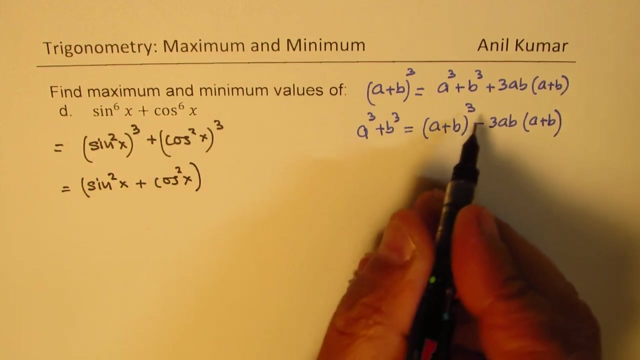 So we are given here sine So cube. we write sine square X, whole cube plus cos square X, whole cube, Right, So A cube plus B cube is A plus B whole cube, So which is sine square X plus cos square X, whole cube. 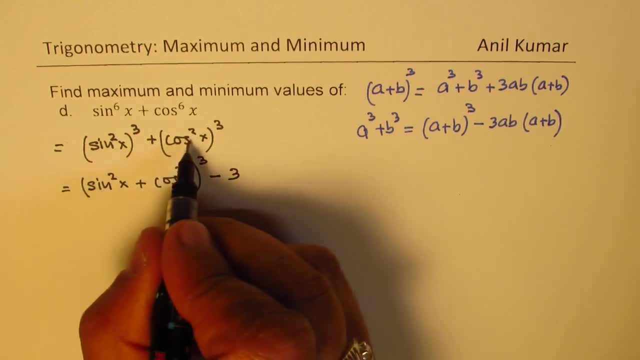 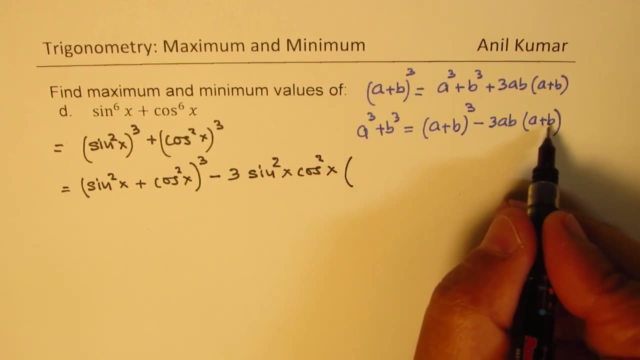 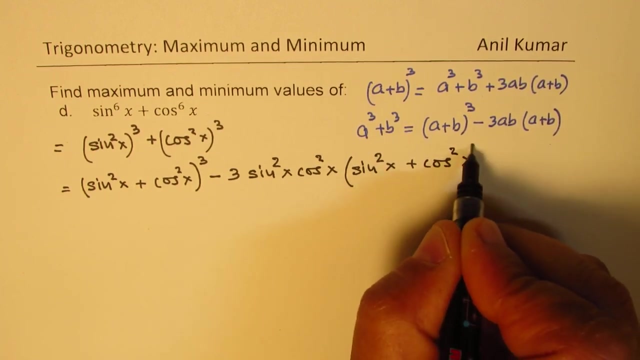 Take away: 3AB means 3 times A and B, which is sine square X, cos square X times A plus B, which is 3AB sine square X plus cos square X. clear Now: sine square X plus cos square X is 1.. 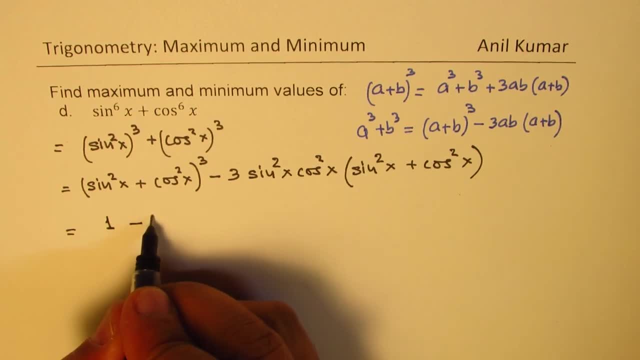 So its cube is going to be 1.. So we get 1 minus 3 times sine square X cos square X. Is that clear to you, Correct? So it is 1 minus 3 times sine square X cos square X. 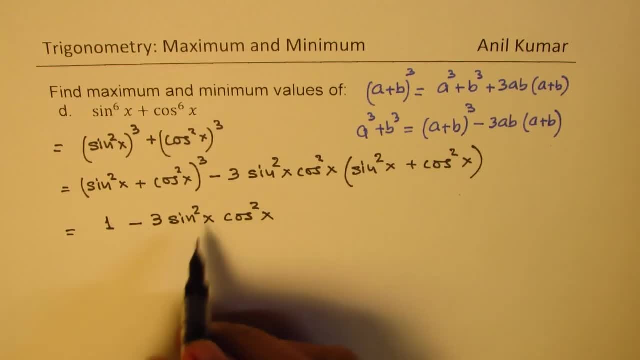 Now for the maximum value. this could be 0, right. So so we have now, for here we have maximum When 3 sine square X, cos square X is equal to 0.. So the maximum is equal to 1 minus 0, which is 1.. 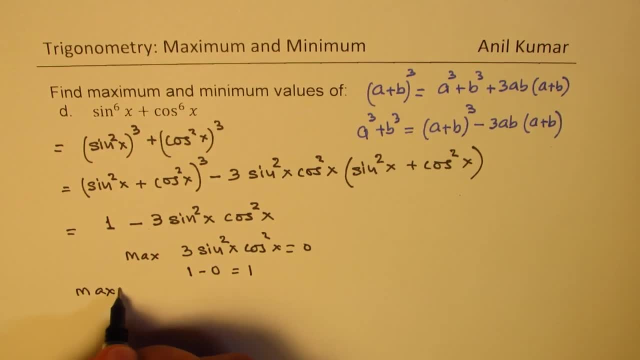 So we get maximum value of 1, right. So maximum is 1.. Now how about the minimum? For the minimum value, this could have 1 over 2, whole square right. So that is what we figured out in the very beginning. 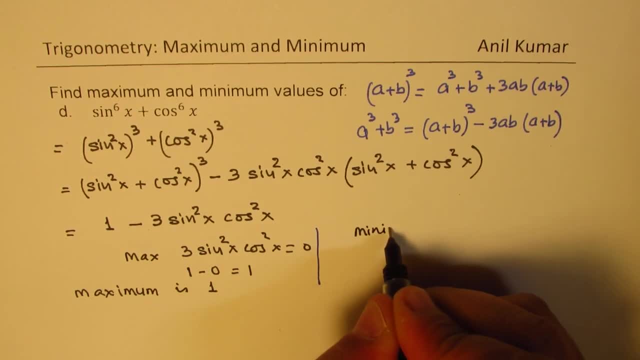 So for the minimum value it will be 1 minus 3 times half square right, Or it is equal to 1 minus 3 times 1 over 4, or it can be written as 4 minus 3 over 4,. 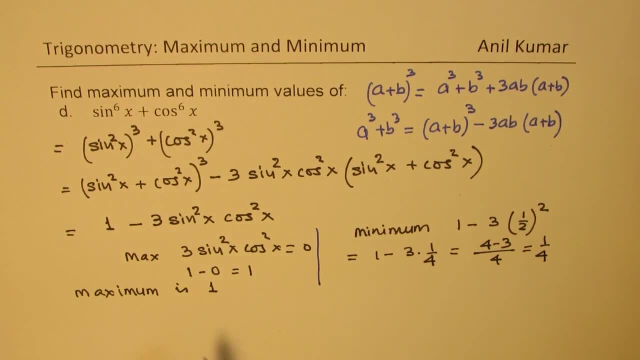 which is 0.. which is one out of four, correct? so the minimum value for this particular function is going to be one fourth right. so now we know that this function, sine to the power of six x plus cos to the power of six x, will be in between one four and one, correct? so that is how we are going to get the